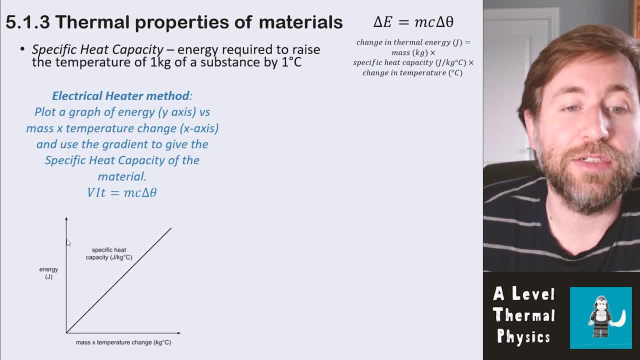 is an electrical heater method. You basically are going to plot a graph of energy on the y-axis and mass times, temperature change on the x-axis, so you get specific heat capacity as the gradient of the graph. Now that uses the idea that the electrical energy is supplied, which is VIT. 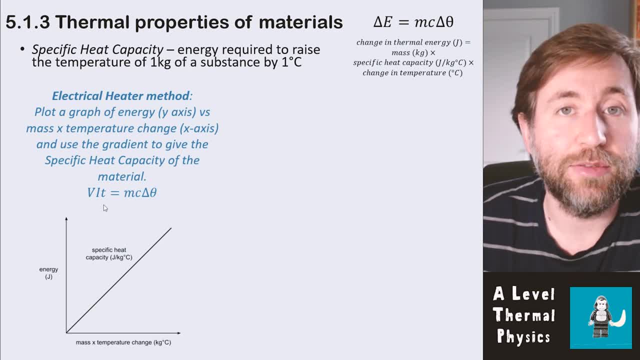 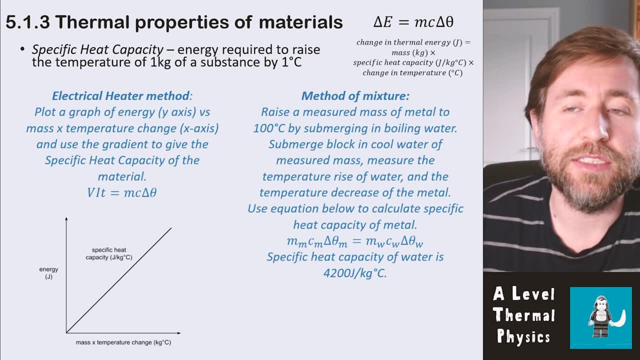 potential difference: times, current times, time, power times. time is equal to the change in thermal energy. There's another method, which is called the method of mixture. Essentially, what you do with this is you raise a mass of metal, a metal block, to 100 degrees Celsius by leaving it submerged in some 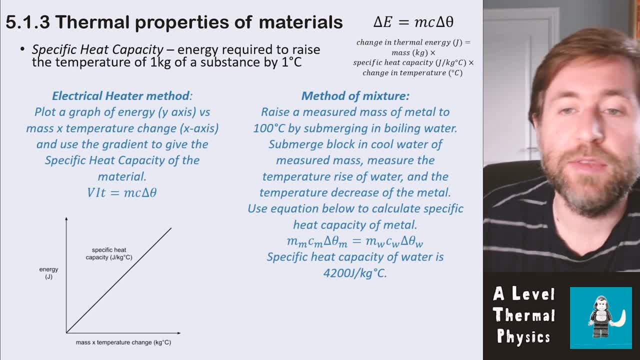 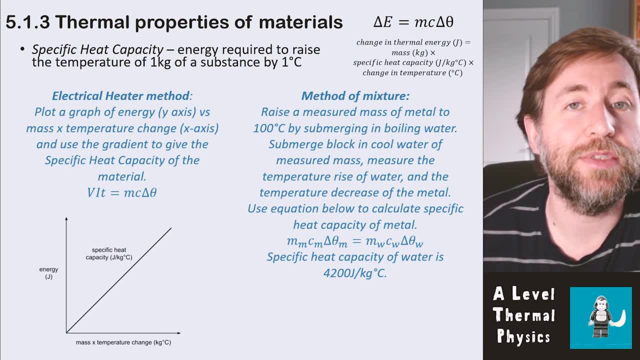 boiling water. So it's going to reach thermal equilibrium with the boiling water. Then you submerge that block in some cool water and you have measured the mass and the starting temperature of that water and you measure the temperature change of the water. You measure the final temperature. 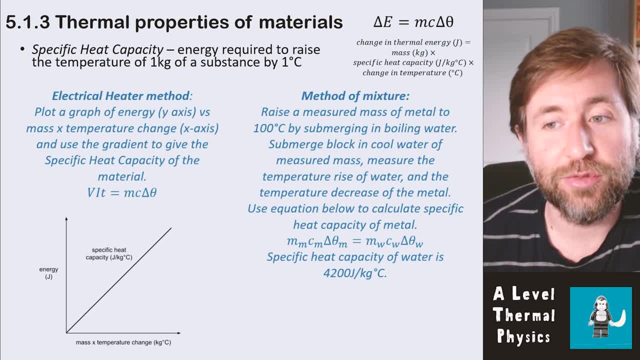 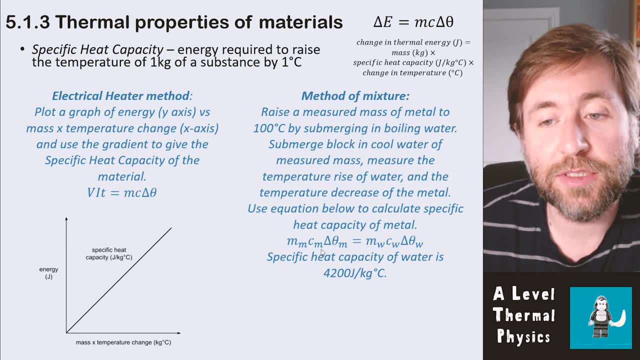 and you work out the temperature change and you also therefore measure the temperature decrease of the metal. You then use the equation below To calculate the specific heat capacity of the metal. So the energy change for the metal once it's submerged in the water is this left hand side and the energy change for the water once the metal 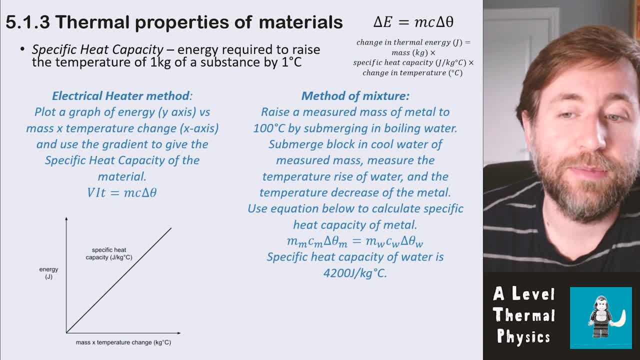 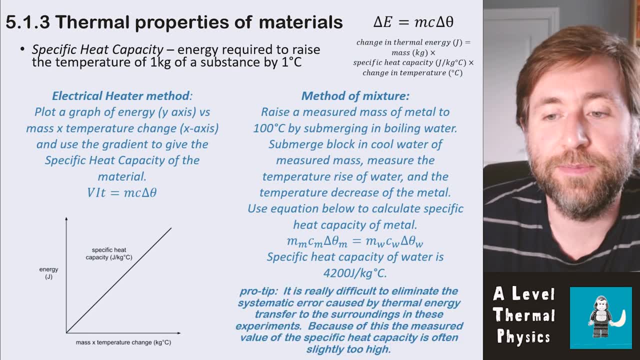 is submerged and they've reached thermal equilibrium again is on the right hand side And you use the value of specific heat capacity of water, which is known as 4200 joules per kilogram per degree Celsius. It's a really difficult one to eliminate systematic error in either of these two practicals. 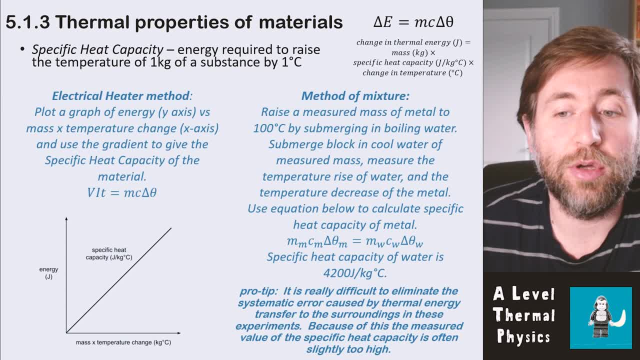 and that's because there's always going to be thermal energy transferred between the block and their surroundings. In this case, they're normally hotter than the surface, so they're going to be warmer than the surface and they're going to be warmer than the surface and they're going to be. 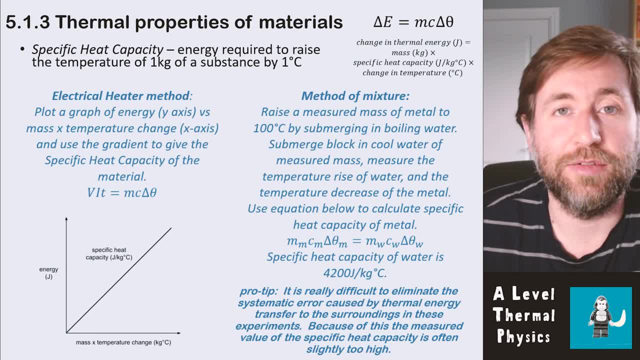 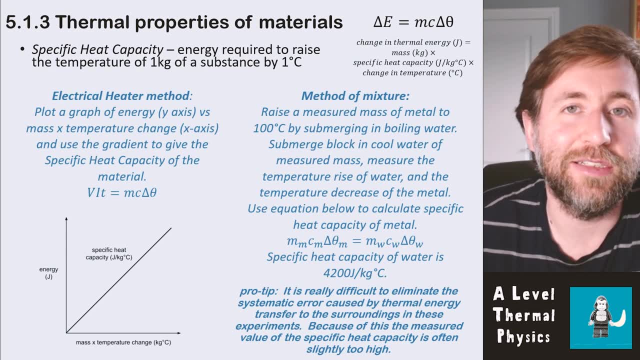 warmer than the surroundings. So you're actually losing energy. you're actually heating the surroundings as well as heating the block, And for this reason you normally get, with these two experiments, a slightly higher specific heat capacity than you're expecting. Another thermal property of materials is specific latent heat. There's two specific latent heats. One is for 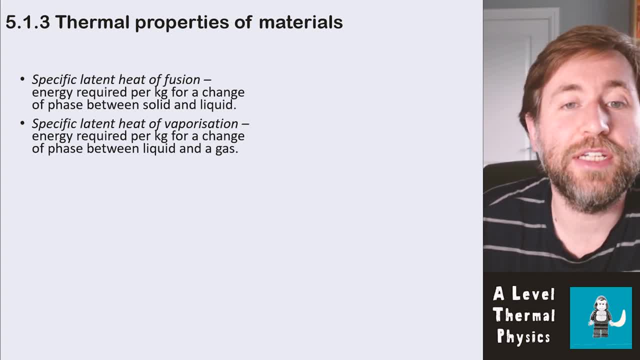 fusion, and that is energy required per kilogram for a change of phase between a solid and liquid, and specific latent heat of vaporization, which is the energy required per kilogram for a change of phase between a liquid and a gas. Now it doesn't matter whether we're going. 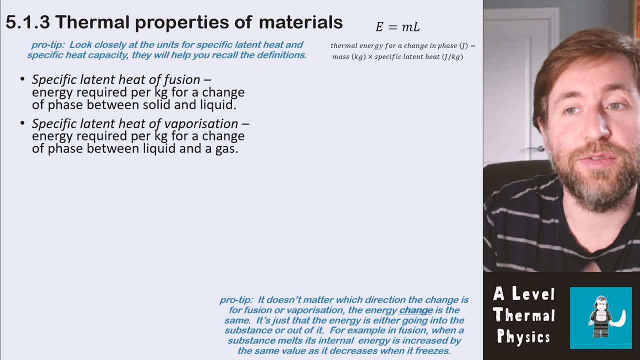 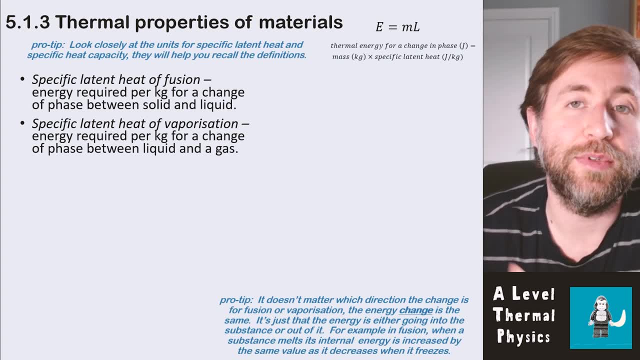 between a gas and a liquid or a liquid and a gas. it doesn't matter which direction it is. the energy change is the same. it's just whether energy is going in or energy is coming out. So, for example, in fusion, when a substance melts, its internal energy is increased by the same value as it will. 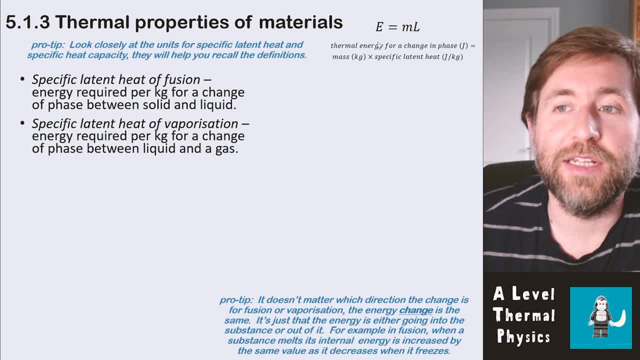 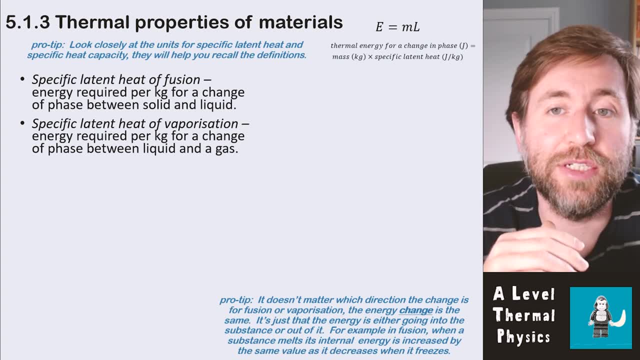 decrease when it freezes. The equation for energy for a change in phase is: E equals ml, so mass times, specific latent heat. Now my pro tip here for this and the previous equation is that actually the units of specific latent heat and the units of specific latent heat are the same, So the units of 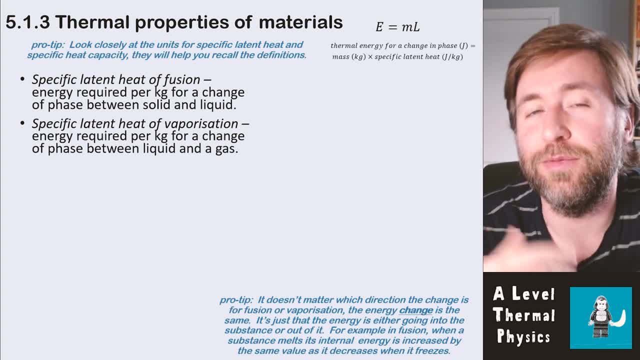 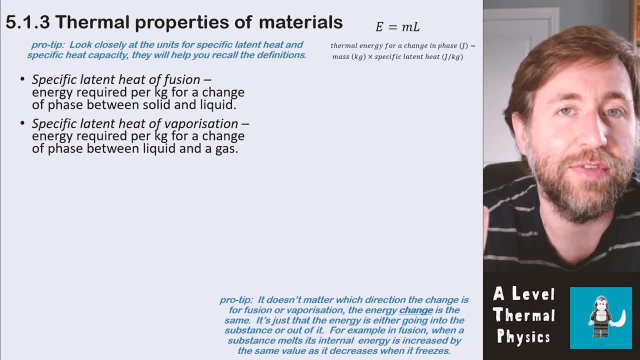 specific heat capacity can tell you exactly what they mean. That's a really important idea in physics, The idea of the units. tell us the dimensions that tell us really what the definition of that quantity is. You need to know a method for measuring latent heat of a material and that's an 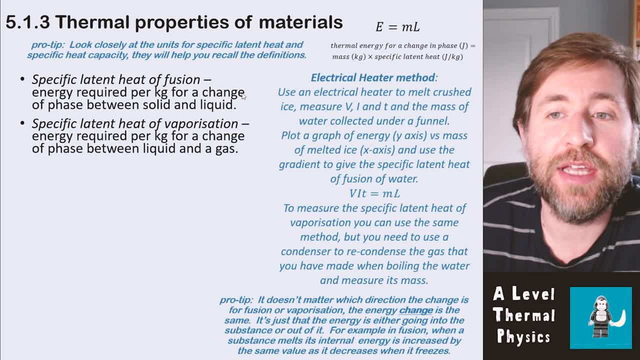 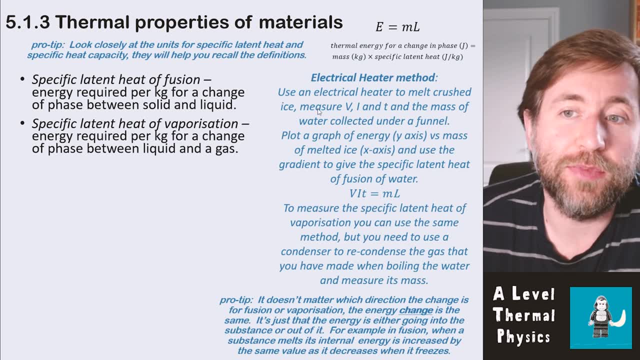 electrical heater method. You need to know a method to measure the latent heat of fusion and of vaporization of water or any other material. really, You can use an electrical heater to melt some crushed ice. You're going to measure the potential difference, the current and the time. 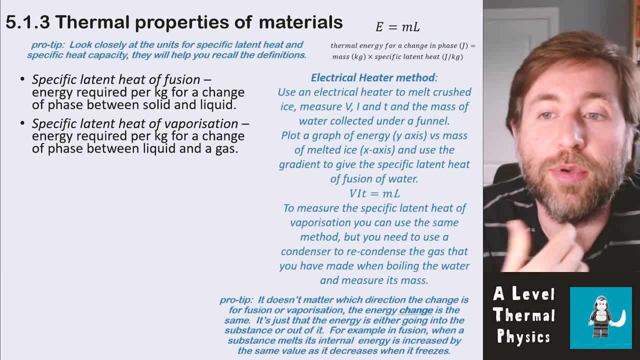 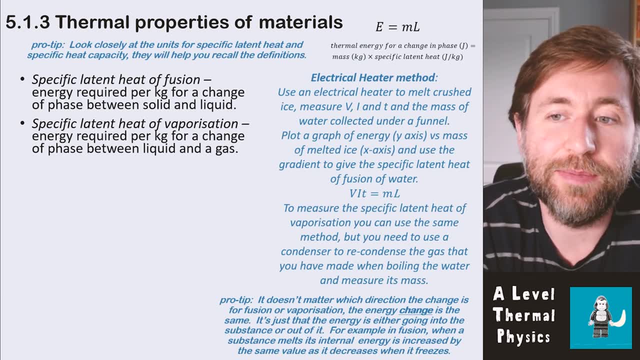 and the mass of water collected by the material. You're going to measure the potential difference of water collected under a funnel and if you plot a graph of energy on the y-axis versus mass of crushed ice on the x-axis, you get a gradient which is the specific latent heat. This is the idea that 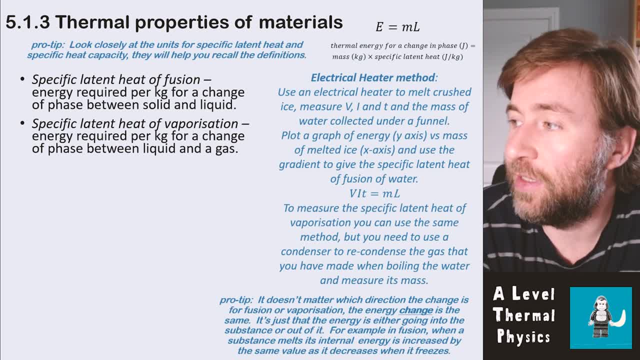 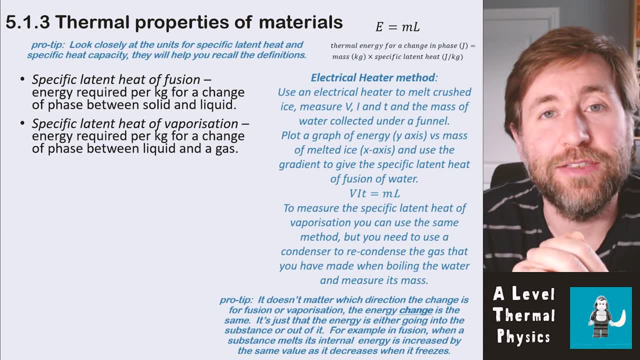 the electrical energy, vit is equal to mass times. specific latent heat. To measure the specific latent heat of vaporization then you need to actually boil some water and collect the vapor that's made. So you actually need to recondense that vapor and then collect that and measure the. 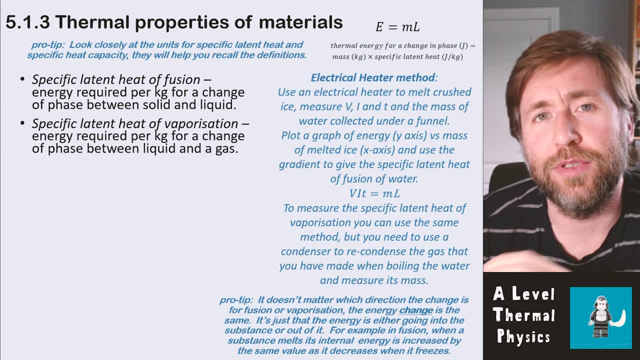 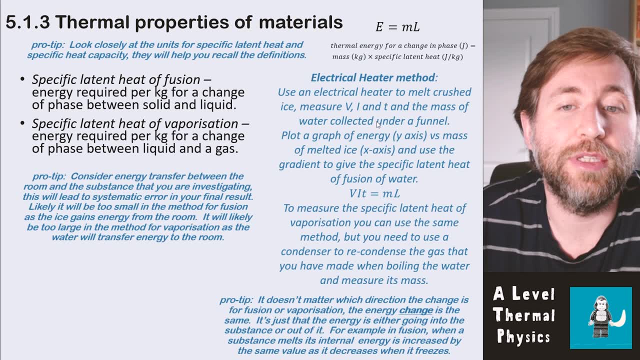 mass of the recondensed vapor. So you're measuring the mass of water, but that's the water that's been accumulated over the history of fusion. that's the mass of vapor. So if you boil that, the ice gets over the energy consumption and you're measuring the mass of vapor. that's the mass of. 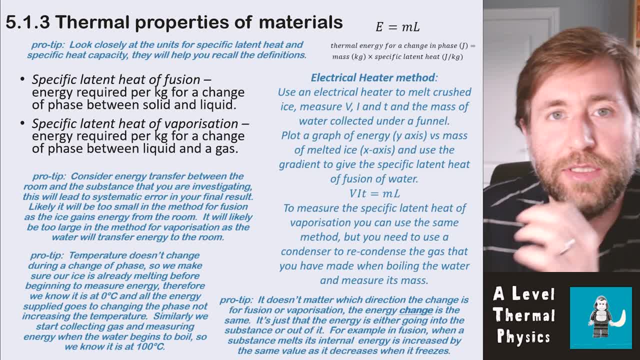 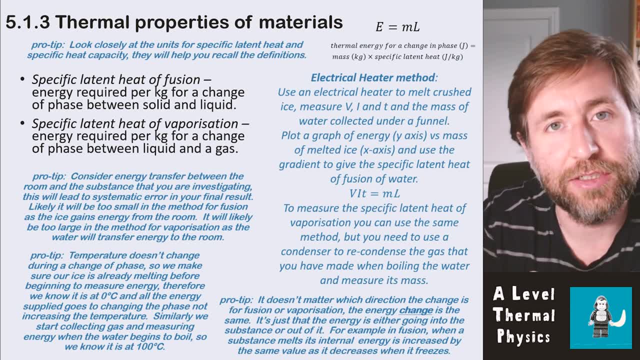 vapor going over the energy consumption. So, for example, you can measure the mass of vapor in the room, if that makes sense. As with the last experiment, you need to consider the energy transfer between the room and the substance you're investigating, and this, again, is going to lead to. 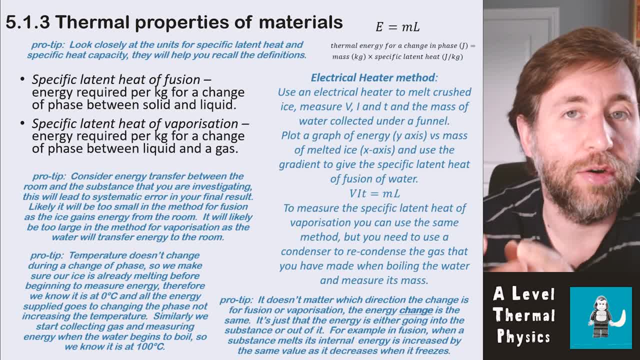 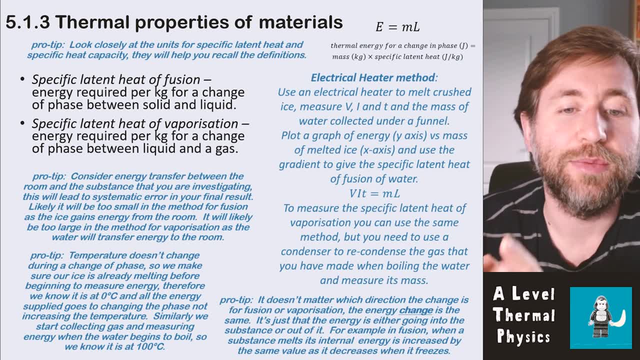 a systematic error in your result. Now, this is likely going to be a little bit too small in the method for fusion, as the ice is going to gain energy from the room. The room is going to transfer energy to the ice, and it's going to be a bit too large in the method for vaporization, as the hot water will transfer energy to the room. 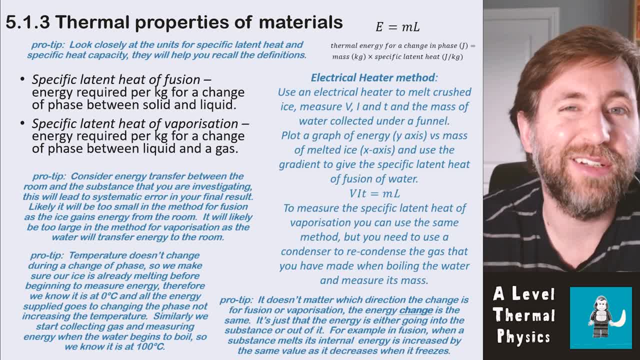 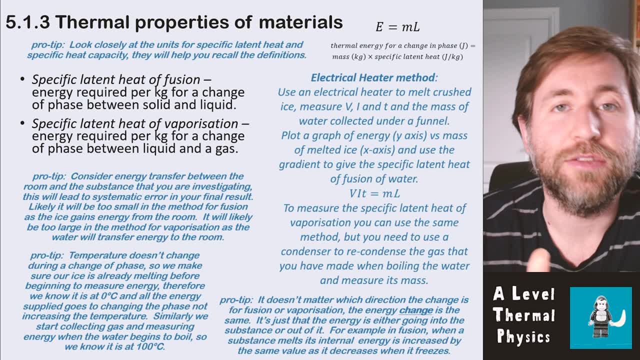 melting before we're beginning to measure the energy. If you pull ice straight out of the freezer, it'll likely be somewhere like minus 20 degrees celsius, and you actually want to know that it's at zero when you start the experiment. So you crush it and let it begin to melt, dripping off any